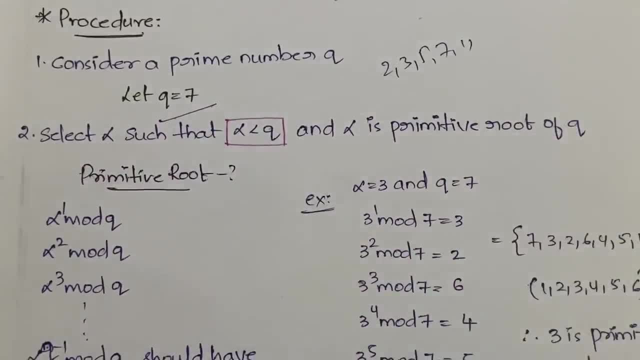 the value of q is 7. here, in the second step, what you have to do is you need to select the value of alpha. alpha is called as the primitive root of the value of the prime number which you are taking. so here the prime number which you have taken is represented with q right. so alpha is the primitive. 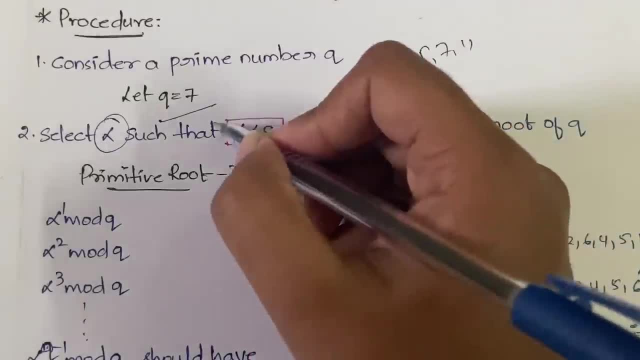 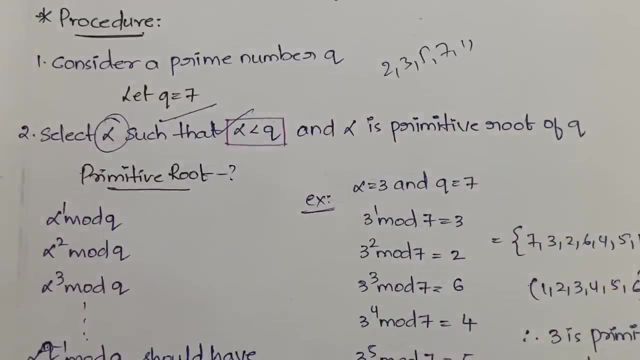 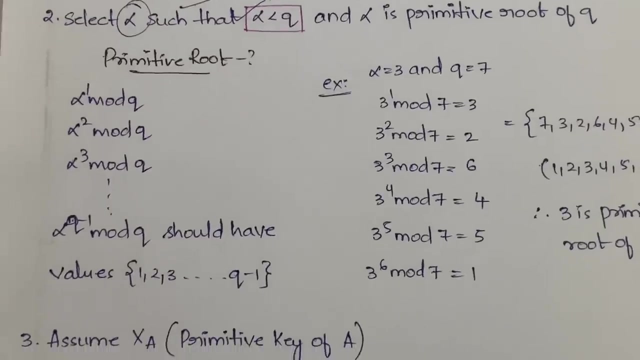 root of q and also also alpha should be less than q. i'll explain you what primitive root is, don't worry, got it. so you have to select alpha such that alpha is less, thank you. and also alpha is primitive root to q, got it? so how do you do that? first of all, primitive root is nothing but. 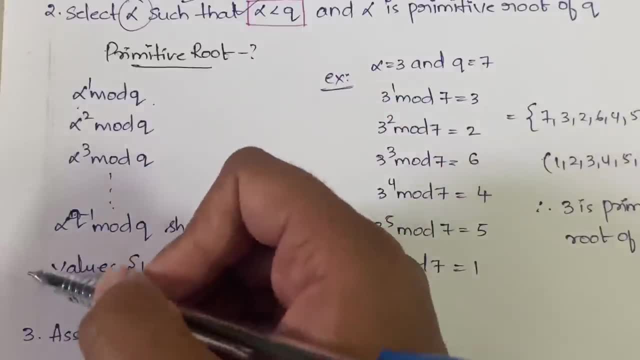 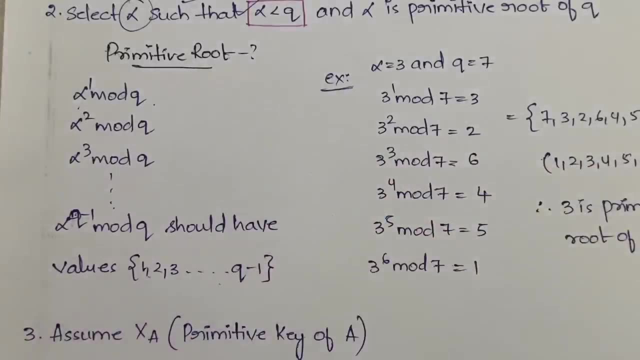 alpha power 1 mod q, alpha power 2 mod q and so on. up to alpha power q minus mod q should have the values in 1, 2, 3 and so on, up to q minus 1. don't get confused. i'll explain you with example. 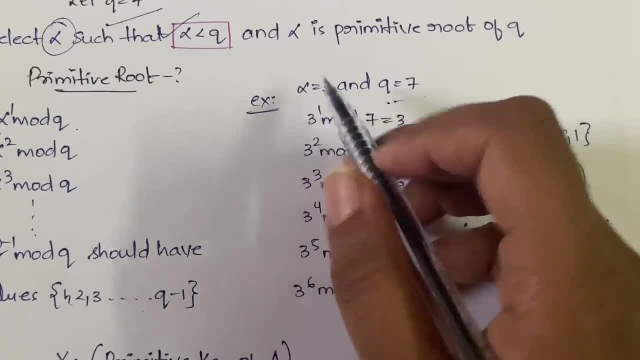 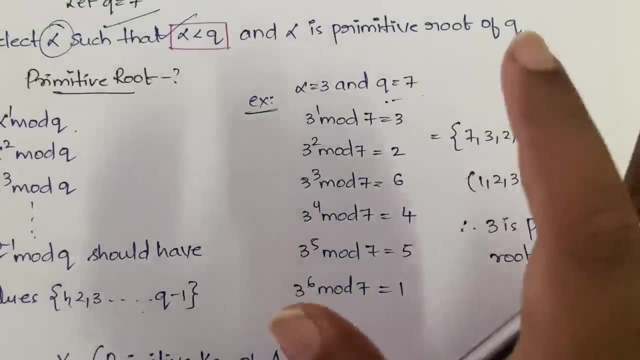 so here, what is the value of q 7 and alpha value? you can take anything but two. you have to keep on checking. first take one and check first, then take two and check, or then take three and check one. do no, don't go with one, because one power, one is one, one power. 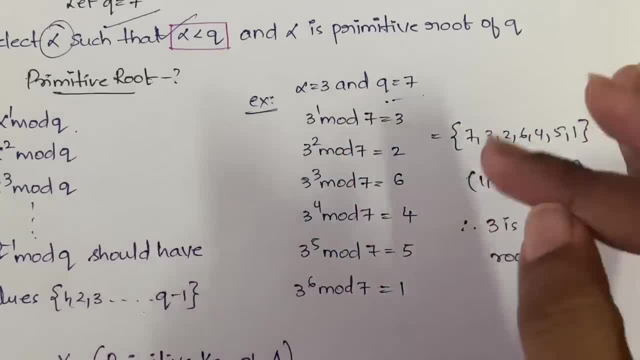 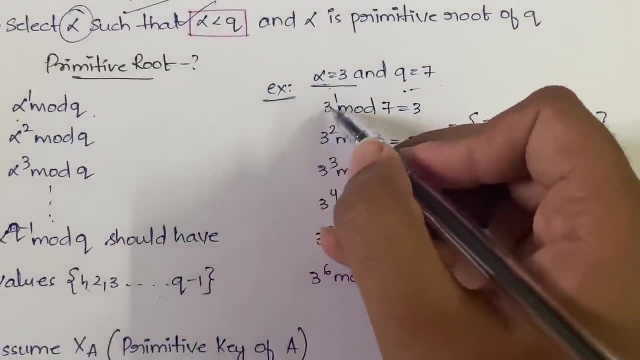 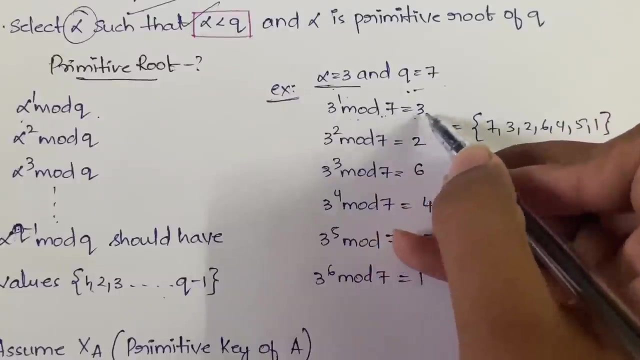 two is also one. one power. three is also one. go, don't go with one, two, three, four, five, like that. you keep on checking. so let us start with. so let us take three here, okay. so three power one mod seven, because q is seven, right? so alpha power one mod q. so three power one mod seven. what is the value? three, 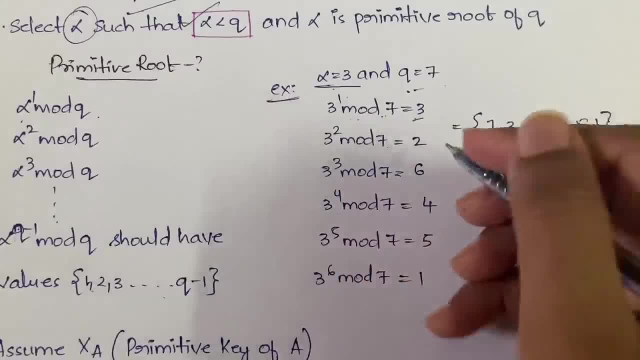 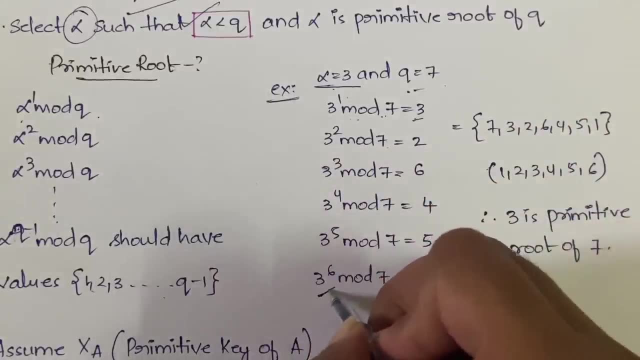 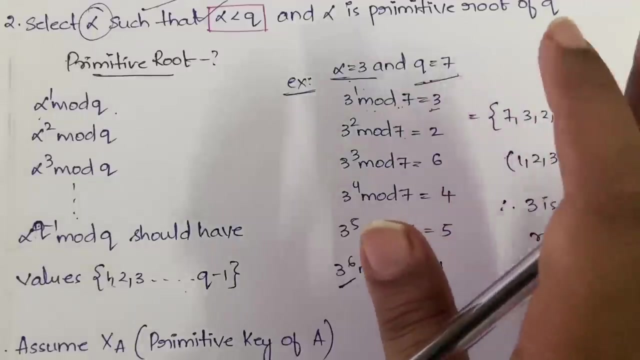 three power, two mod seven. what is the value? nine mod seven, two. a remainder right: 2. so 3 power 3, 3 power 4. so like that. up to which power you have to do? up to 6, why, up to q minus 1 you have to do alpha power, q minus 1. what is the value of q here? 7, 7 minus 1 is 6. 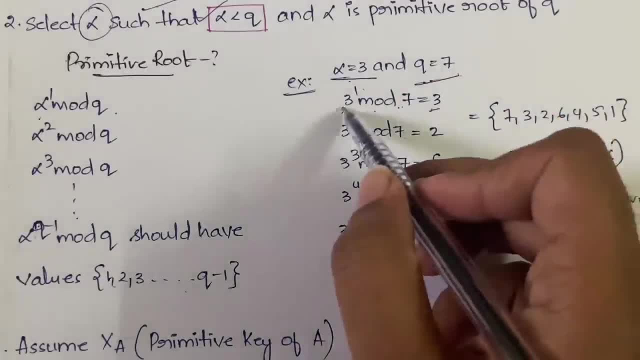 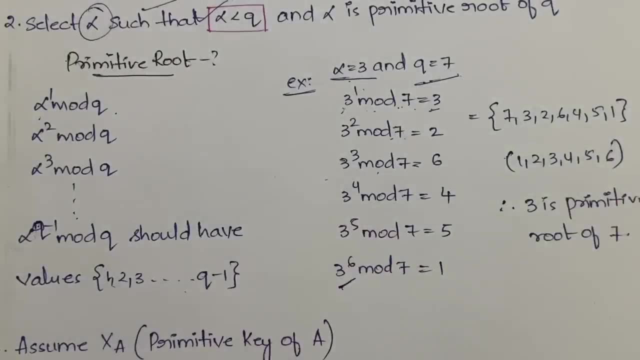 so up to 3 power 6, you have to do. okay. so 3 power 1 mod 7, 3 power 2 mod 7, 3 power 3 mod 7, like that. up to 3 power 6 mod 7, you have to do. got it now. after doing you need to check the values. 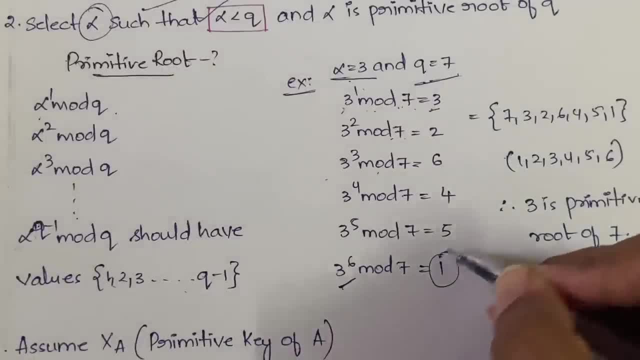 so you here, you have 1, 2, 3, 4, 5, 6, right? so you have all numbers from 1 to 6, that is, you have all numbers from 1 to q minus 1 in the range, right? so when you list out all these reminders, 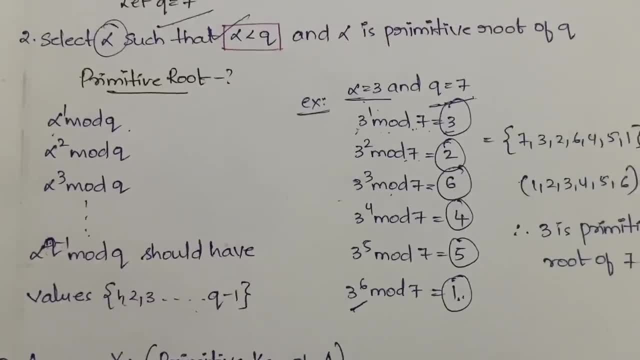 you need to get all the numbers from 1 to q minus 1, that is, from 1 to 7 minus 1, that is from 1 to 6. you got it right. so that is why alpha is the primitive root of q, that is, 3 is primitive root of 7. that is what this means, right? so in the 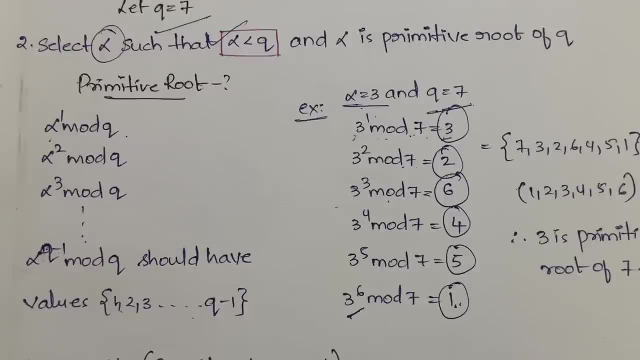 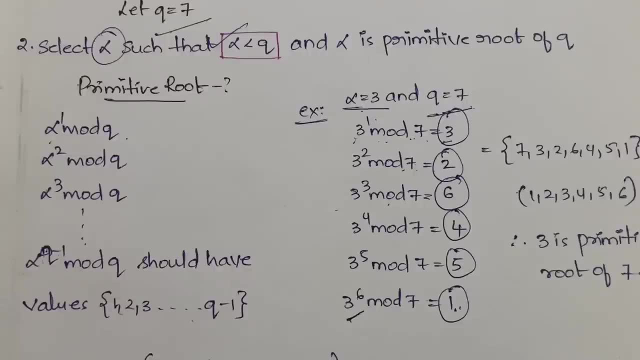 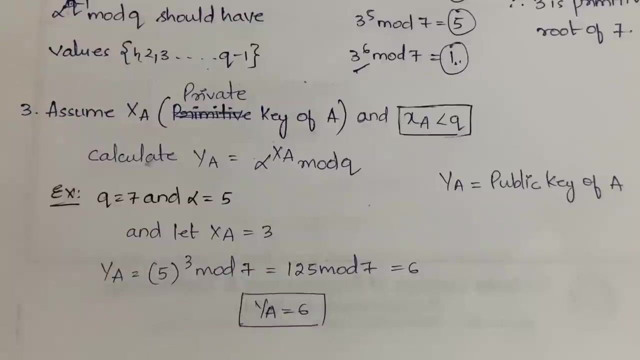 second step, what you have to do. you need to select alpha, which is nothing but the primitive root. primitive root means this one. you need to, it has to follow this sequence, it has to follow this rule. okay, so next, in the third step, what we will do, let us see now. so now we are done with selecting. 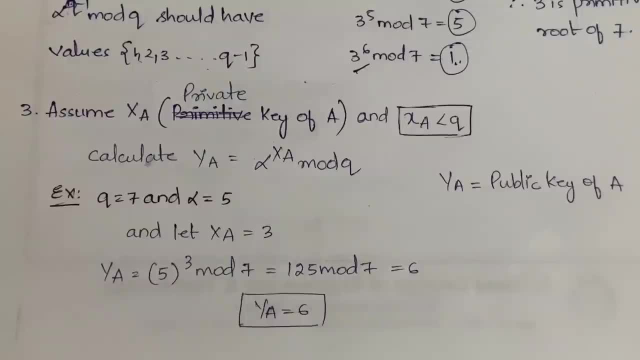 q and alpha. right, q is nothing but it is a number and we have taken that as 7 and alpha is. we got the primitive root, got it. so now, after that, in the third step, what you have to do is you need to assume the value of xa. now, what does this xa? 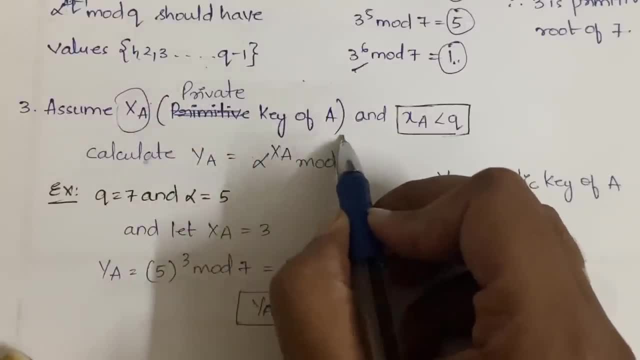 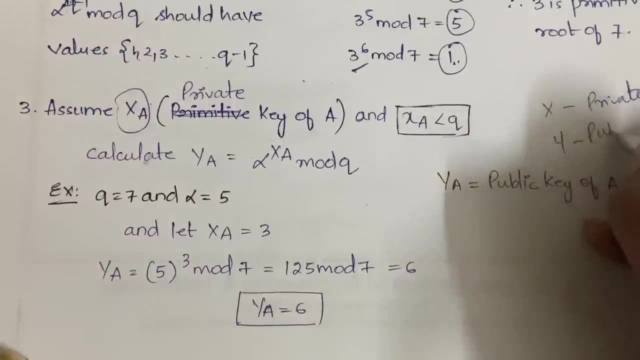 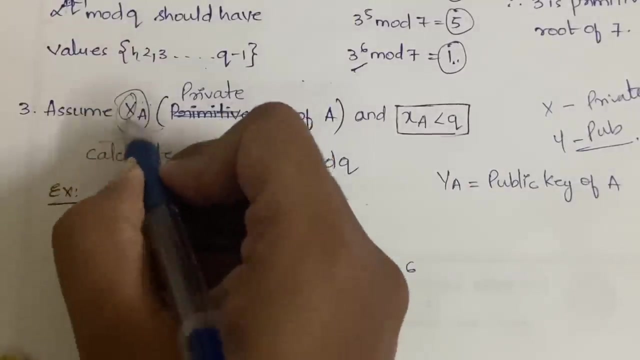 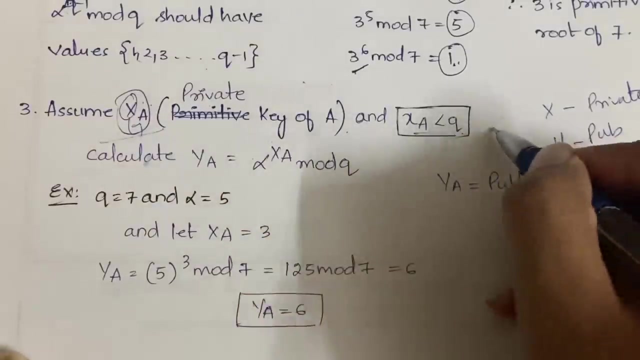 means private key of a. okay, so x means private, y means public. for a or b, whatever it is, x means private, y means public. remember that. so here xa represents the private key of a. okay, private key of a. and also xa should be somewhere, something which is less than q. what is the value of q 7? so 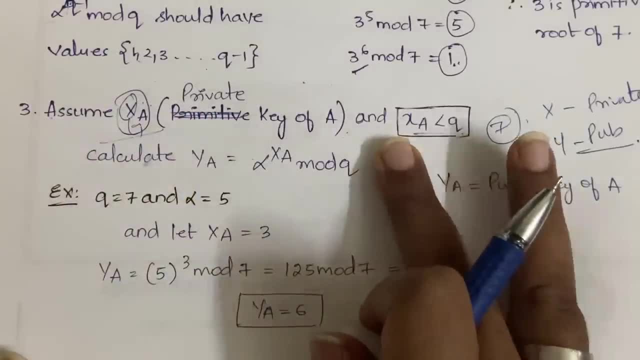 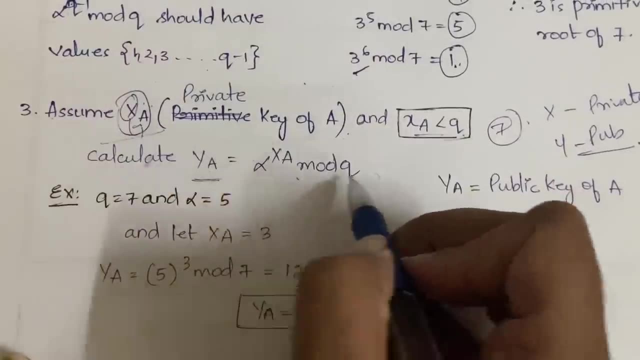 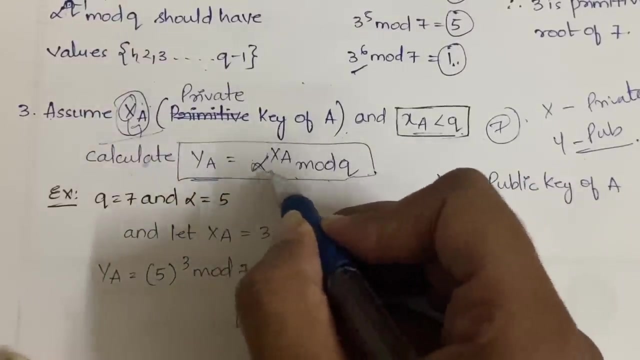 you need to assume the value of xa such that it is less than 7. got it. now you have to calculate the value of ya using a xa value. you need to calculate the value of ya. how do you do that? ya is equal to alpha power, xa mod q. you already know what alpha 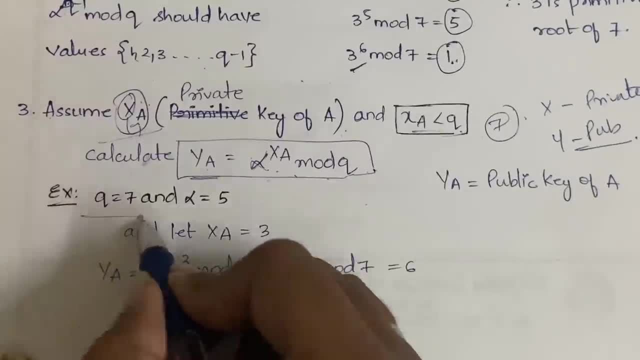 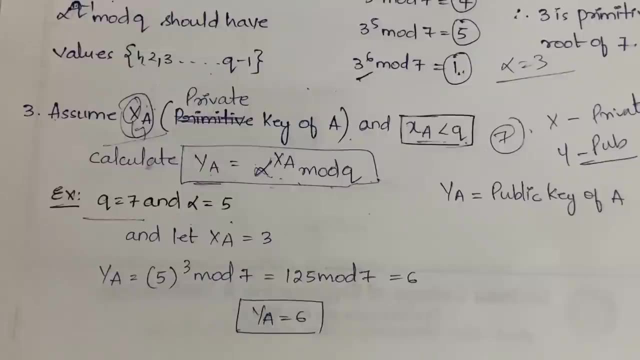 is. alpha is a primitive root of q, right? so we have taken q is equal to 7 and alpha is equal to 5. actually we got alpha is equal to 3 here. but you can take anything. check with phi also whether phi is satisfying or not. if phi is satisfying, you can take alpha as phi as well. 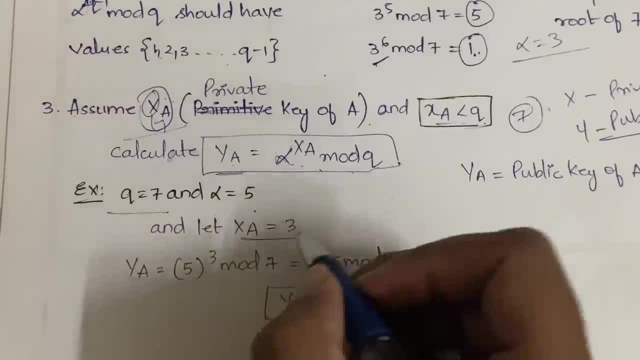 so we have taken phi and we have assumed xa to be 3. why xa is 3? you have to assume any. you can assume anything which is less than 7. you can take 4, 5, 6, whatever it is you can take, but always try. 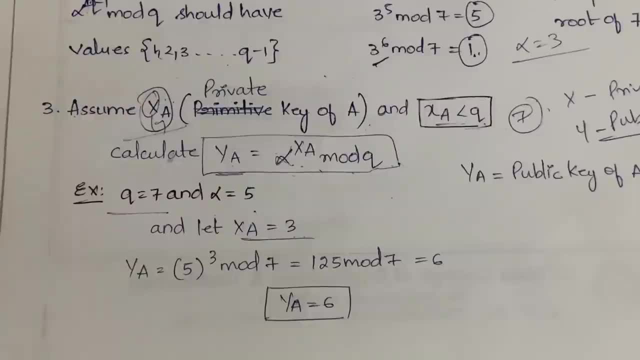 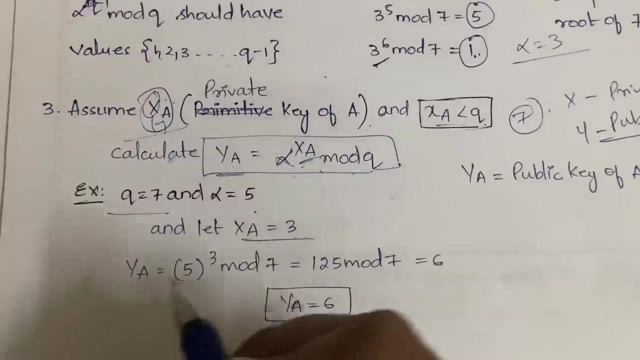 to select um minimum value because you have to do the power operation here, right, alpha power, xa. you are doing so. if you choose a really very big number, then it becomes more complicated. so choose that small number in the sense, not just like 1, 2 or 3 is the best. so xa is equal to 3 and 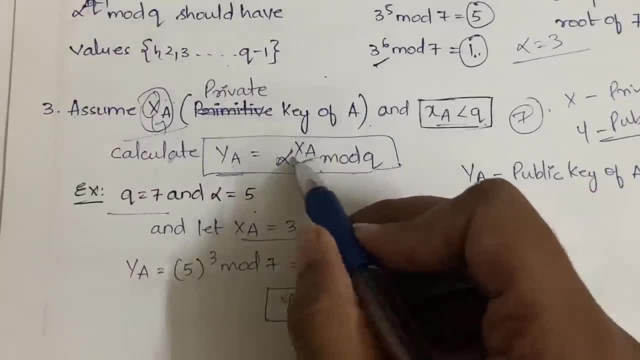 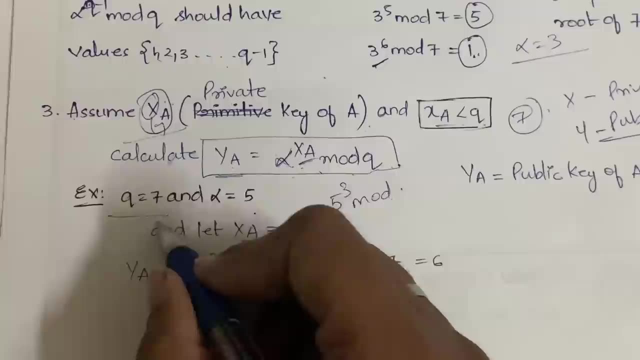 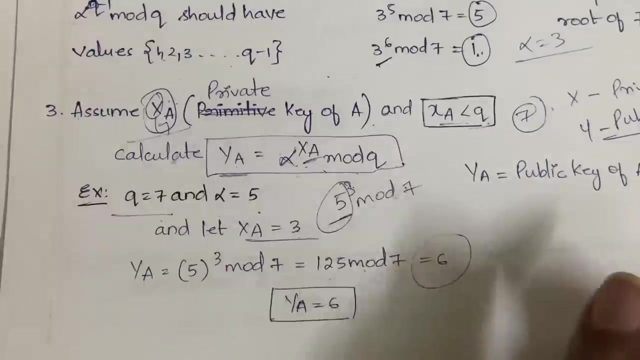 ya, is equal to 5. power 3 mod 7 alpha. power xa mod 7. right alpha is 5 and power xa xa we have assumed as 3 and mod q is nothing but q is 7 and 1, 5, 5. power 3 means 125, 125, mod 7 means 6. okay, so, 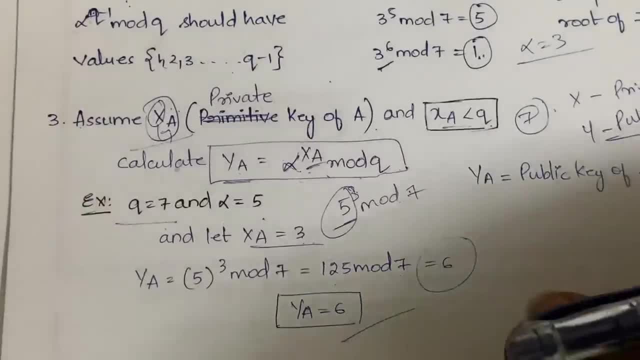 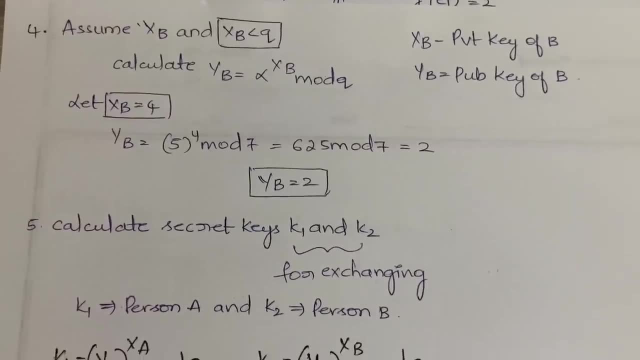 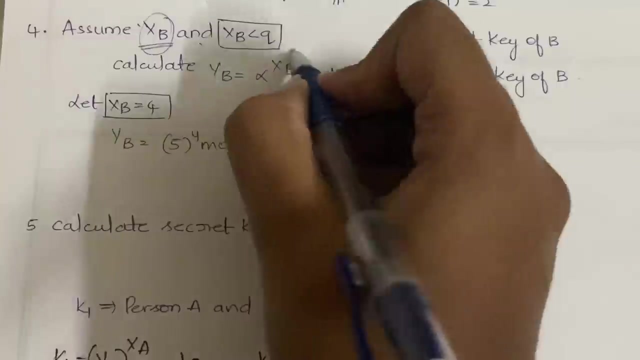 now, we got the value of y a. got it. now, after getting the value of y a, what you have to do? you need to find out the value of y b. how do you find out the value of y b? in order to find out the value of y b, you have to assume x b. okay, x b, and x b also should be less than q. the same. 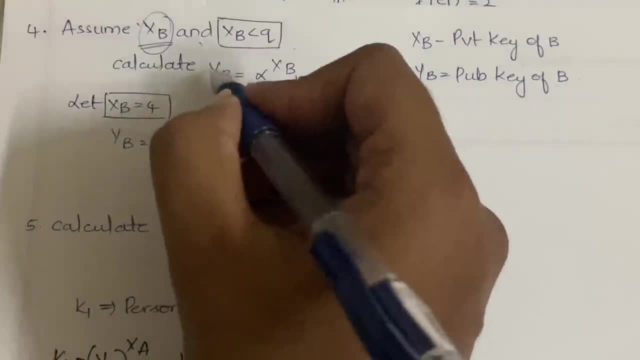 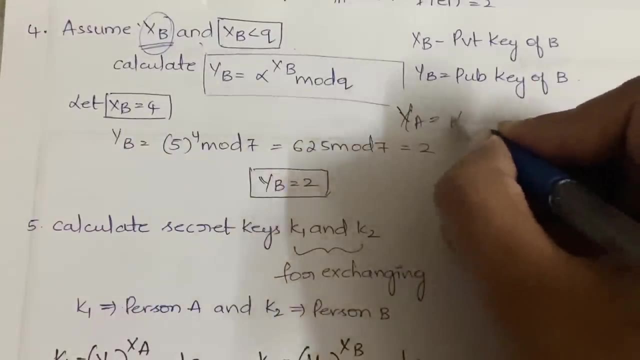 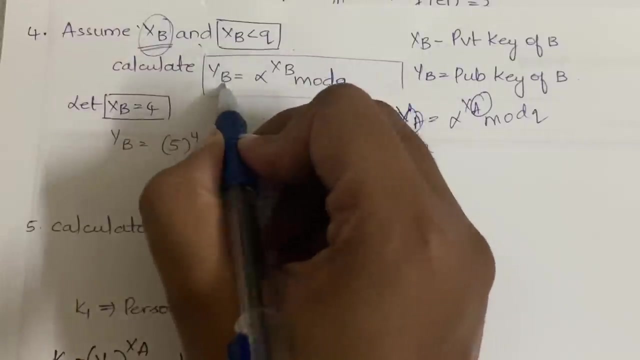 constraint. here also it goes, and you need to calculate the value of y b as alpha power x b mod q. in case of what is the formula for y a? it is alpha power x a mod q, right? so for a you're taking a, got it. so you need to calculate y b, which is equal to. 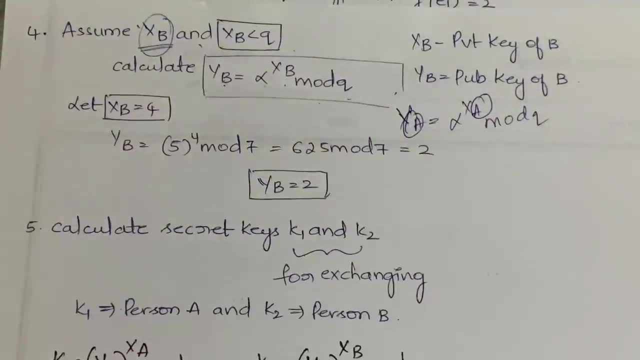 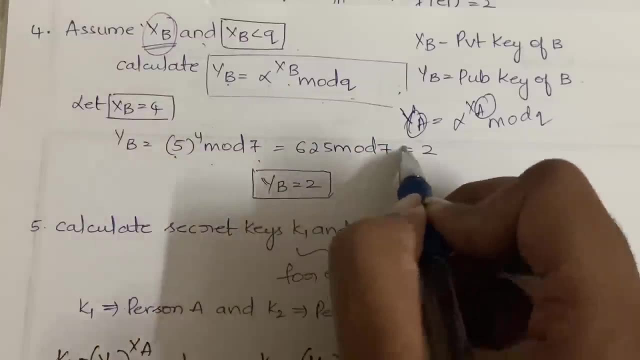 alpha power x b mod q, and let us take as x b as 4 we have. we have to assume x b it can be anything which is less than the value of 7, right? so y b is equal to 5 power 4 mod 7, which is 625 mod 7. you. 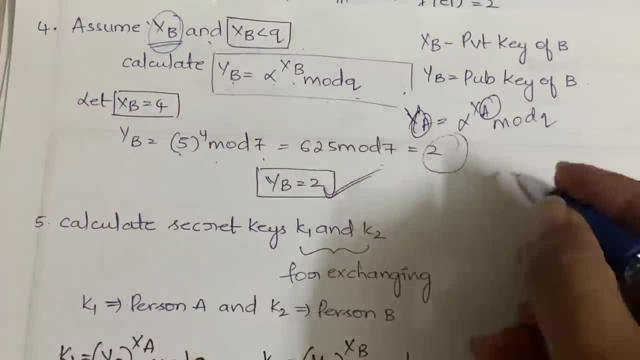 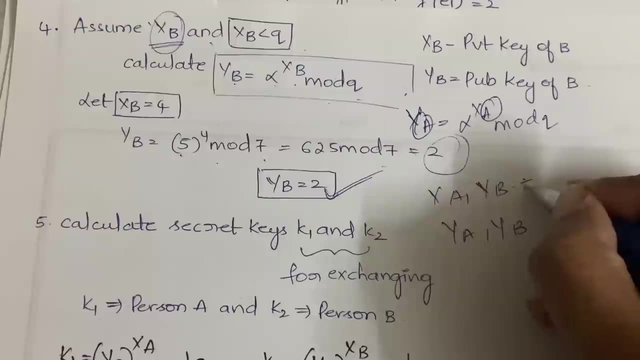 get 2 right. so now you got the value of y b as well. now you have the value of x a, x b, y a and y b. what is the value of x a? it is, we have assumed it as 3. and what did we get? the value of x b? sorry, we have assumed the value of x b as 4, right? 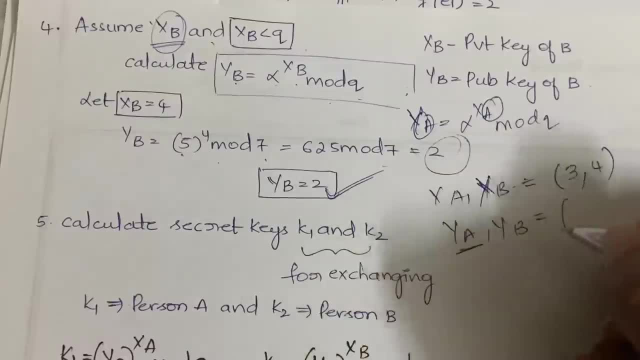 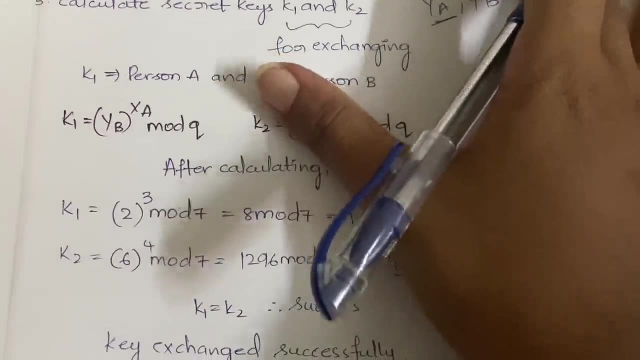 and what did we get? the value of y a on solving, we got it as 6 and y b is 2, so 6 comma 2. so we got the values of x a, x b, y a, y b done. now, in the fifth step, what you have to do is you need to. 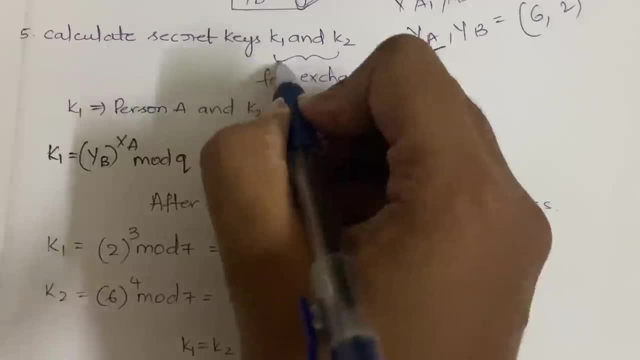 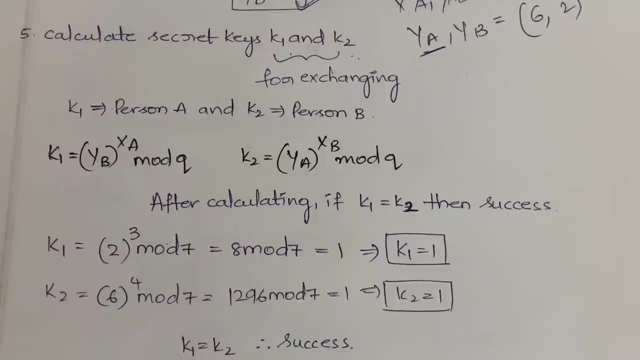 calculate the secret keys k 1 and k 2. so this actually defy hellman algorithm. is what key exchange algorithm, right? so here we are going to check whether the key is exchanged successfully among a and b or not, got it? so how do you verify whether it is? 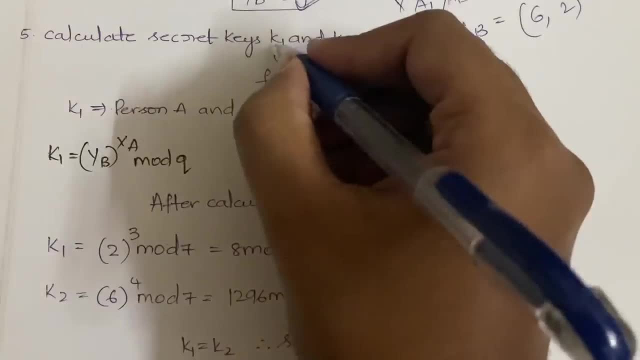 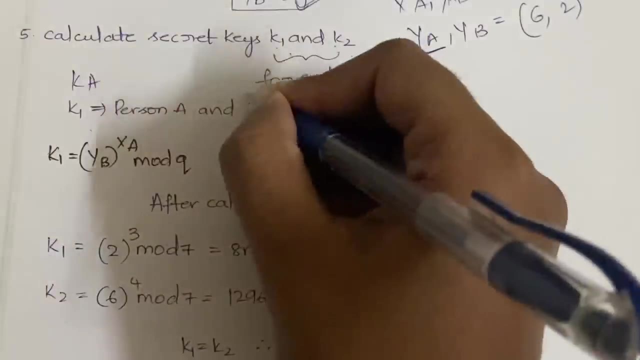 success or not, i'll tell you. so now you have to calculate k 1 and k 2, so k 1 belongs to person a and k 2 belongs to person b. or else, in case of k 1 and k 2, you can take k a. k b also got it, so k 1. 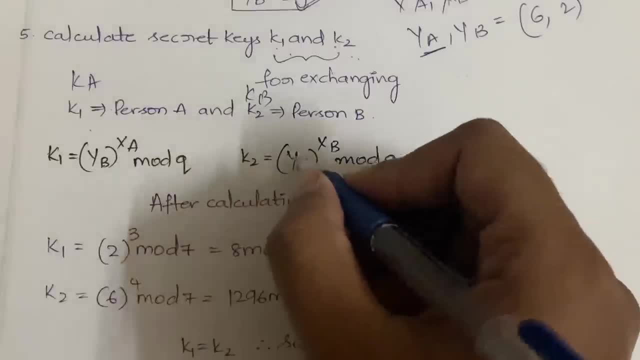 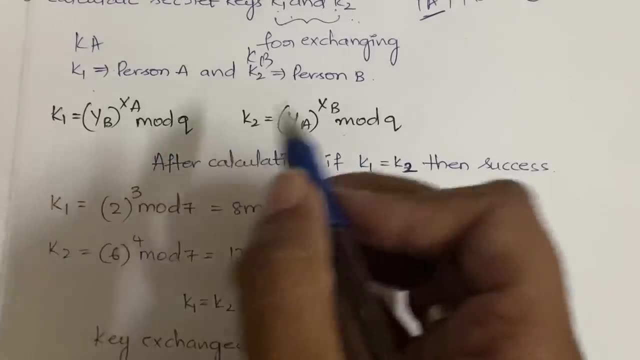 will be equal to y b power x a mod q and k 2 will be equal to y a power x b mod q. right? so you need to use these two formulas and find out the value of k 2. now, what is the k 1 and k 2 value of k 2. 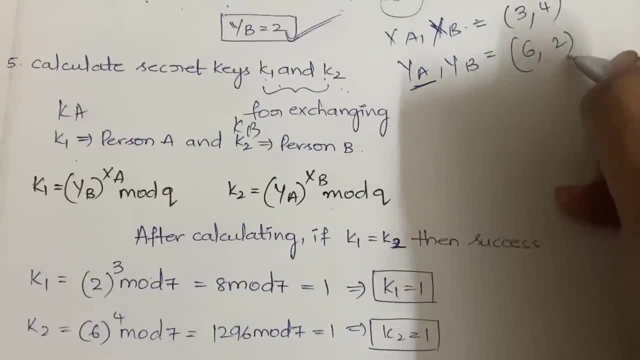 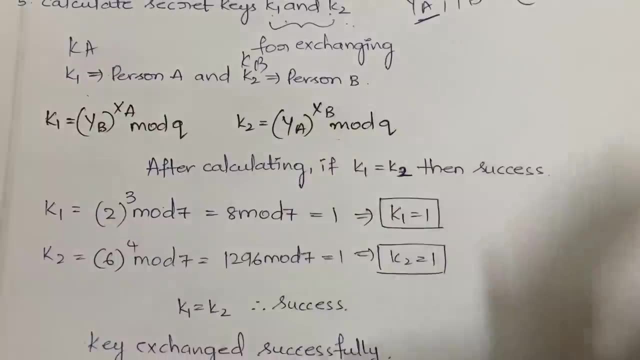 k 1. you know what is the value of y b? it is 2, so 2 power. what is the value of x a, 3, 2 power, 3 mod 7? it's the same: 2 power 3 mod 7, 8 mod 7, which is 1 k 1 is equal to 1. you got okay done now. y a power, x b. 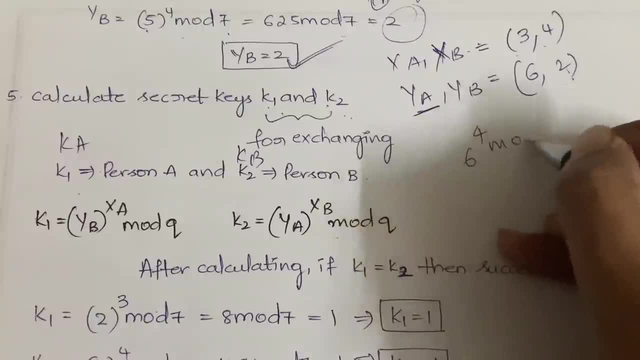 what is y a 6 and what is x, b, 4, 6, power 4 mod 7, 6, power 4 is what? 1, 2, 9, 6, 6, 6 are 36, 36 into 6 is 2. 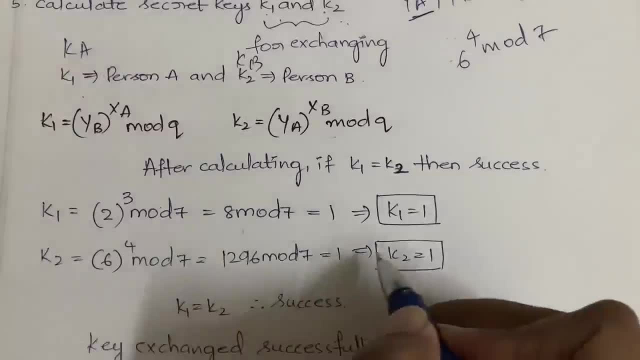 1, 6, 2, 1, 6, 6 into 6 is 1, 2, 9, 6. so we got 1, 2, 9, 6, 1, 2, 9, 6 mod 7. you do again. you get 1. so k 1 is equal. 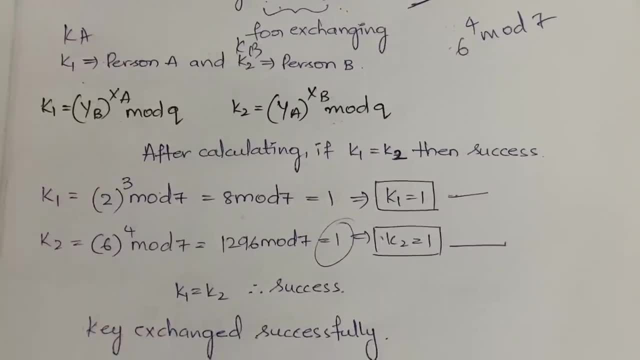 to 1. so what did you get here? both k 1 and k 2 are equal to each other, right? so when both of them are equal to each other, then key exchange is to. e is said to be done successfully. otherwise, no it. it may not be that always. k 1 and k 2 should always be equal to 1. it can be 2 or it can be 3. 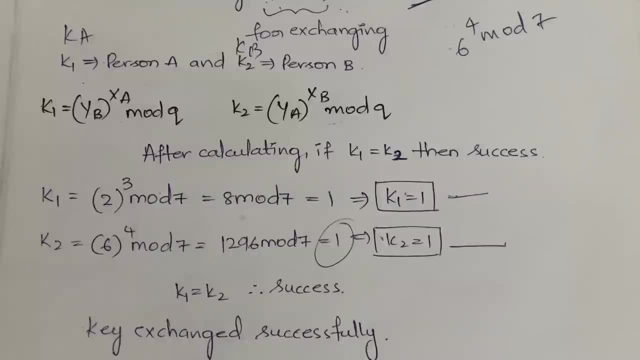 whatever number it is, both of them should be always equal. in that case, you can say that the key exchange is successful, got it. so this is all about the defy helman algorithm in this algorithm you are not. this algorithm is not for encryption or not for decryption. 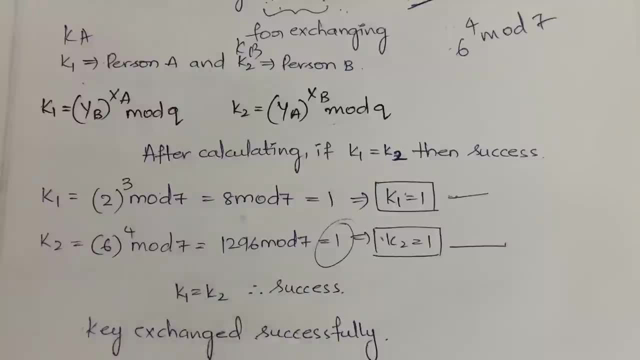 you are not for encryption or not for decryption. you are not for encryption, you are not for doing here. mainly you are doing key exchange. so you exchange the key between the sender and the receiver got it and you will be checking whether key has exchanged successfully or not by value, by 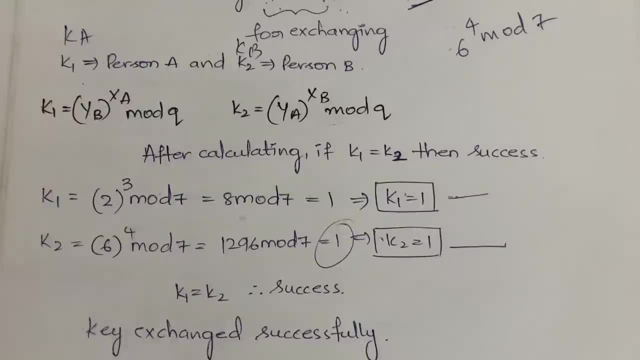 calculating the values of k 1 and k 2. got it. how do you find out the values of k 1 and k 2? by using x a and x, a, x b, y a, y, b, that is, using the private and public keys of both a and b. got it, though this. 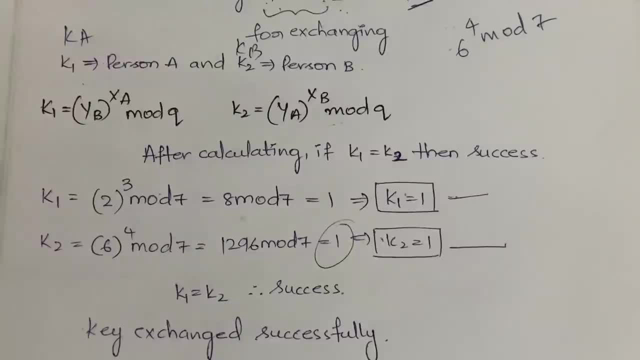 is all about the diffie-hellman algorithm. so this is very, very. i don't say it is very simple, but it is not so hard as well. so this is very simple, but it is not so hard as well. so this is very, very had as well. there are so many algorithms which are more complicated than this.